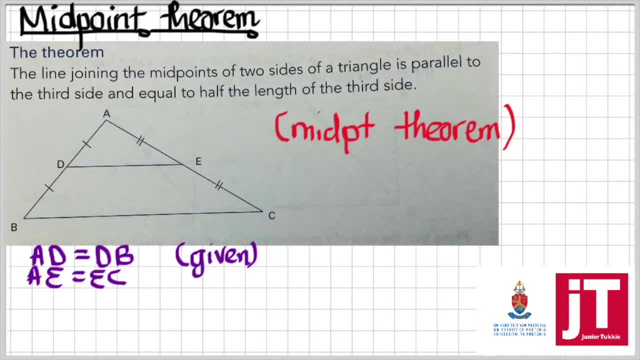 It's marked. And also the side AE is equal to EC. Again, that's another given. You can see that from the diagram as well. We then make a conclusion that the side DE has to be parallel to BC, And the reason for that is the midpoint theorem. 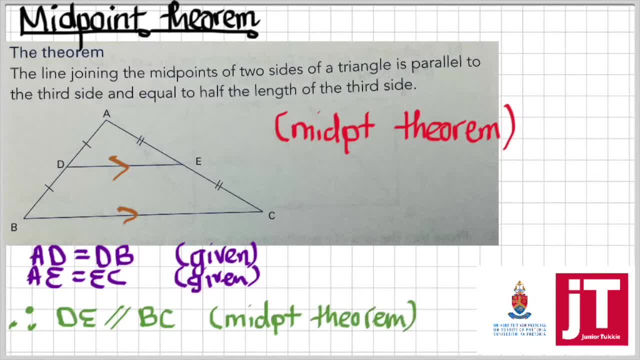 It is the midpoint theorem And I've marked them on the diagram to see that those two sides are parallel. Also, we know that BC is actually two times DE, So I can say BC is also two times DE. Again the same reason. 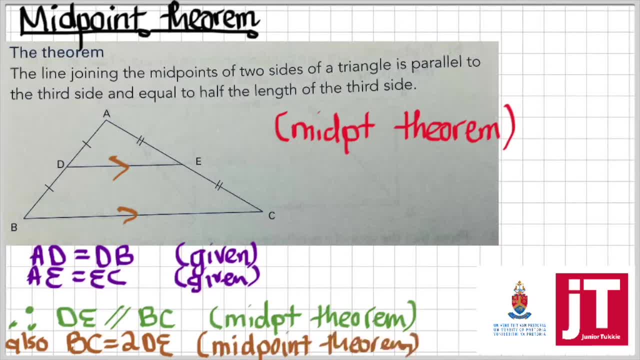 The same reason is the midpoint theorem in full. We move on to the converse of that theorem. So when I look at the converse of the midpoint theorem again, I'm going to make use of a diagram And if you look at the diagram it looks somewhat similar. 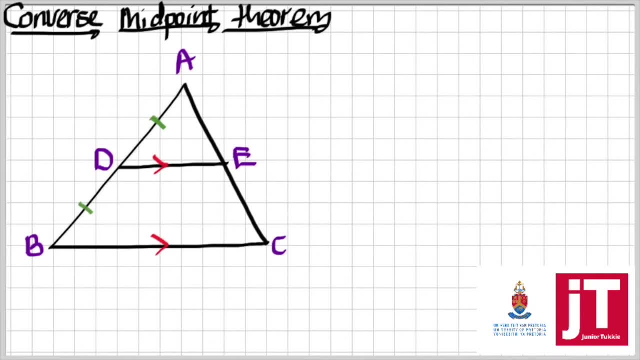 But the difference with this diagram and the previous one is that with this diagram, which deals with the converse, we are already told that the line DE is parallel to the side BC, which we were not given previously for the midpoint theorem. that would form our conclusion. 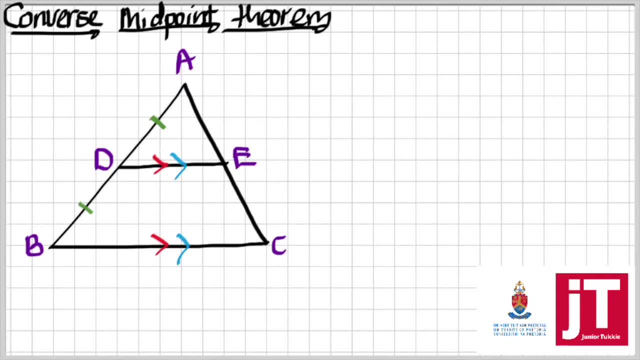 Now, that is a given. What we are not given, however, is that this side here, the side AE, is equal to the side EC. That is not a given. That's what we want to conclude in the end, So I'm going to take off all that. 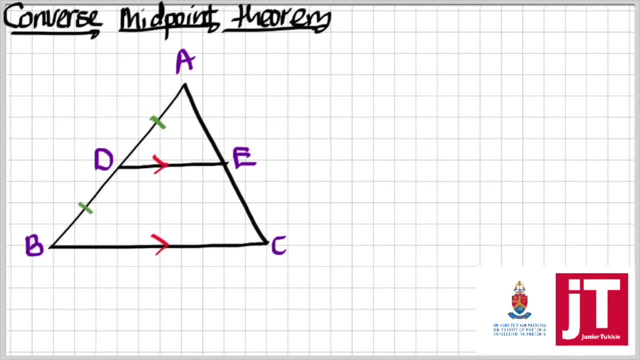 So I just go back to the original diagram. Then obviously I need to state the theorem theorem in words, just like what we did previously. so the converse of the midpoint theorem states that a line drawn parallel to this to a side, from one side's midpoint to the other side, bisects. 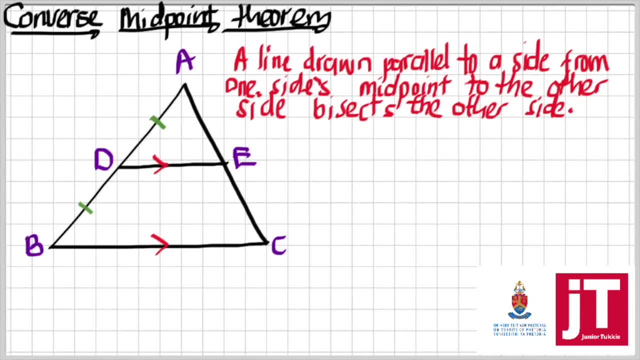 the other side. a line drawn parallel to a side, from one side's midpoint to the other side, bisects the other side. so we are told here, to summarize it, that if there's a line that has been drawn from the midpoint- assuming that the point d is the midpoint and is drawn parallel to the third side-